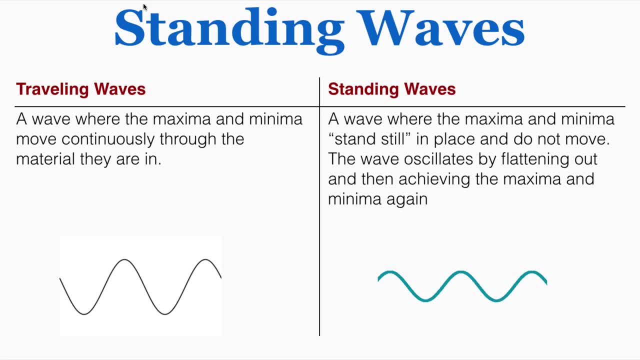 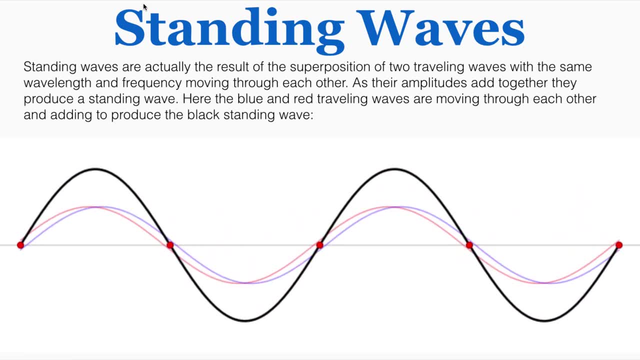 key to understanding a ton of stuff that happens in physics. Standing waves are actually the result of the superposition of two traveling waves with the same wavelength and frequency, moving through each other As their amplitudes add together. following the rules of superposition, they 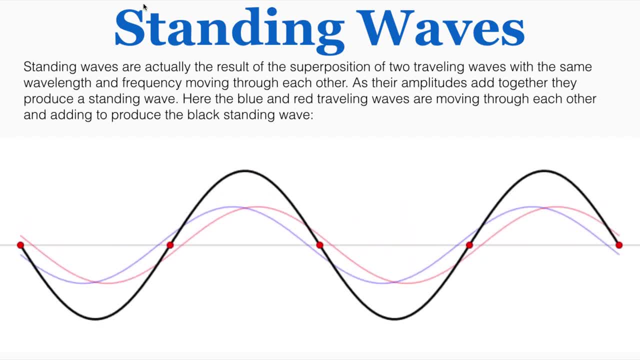 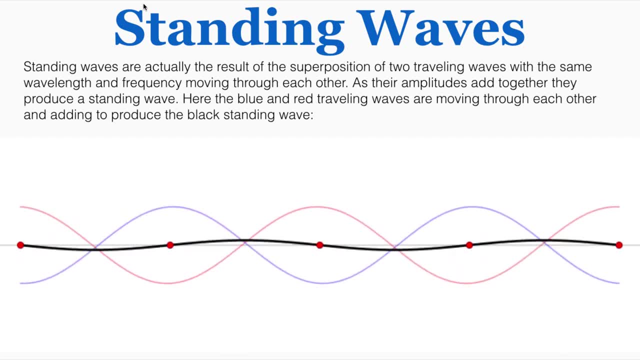 produce a single standing wave. Here. the blue and red traveling waves are moving through each other and adding to produce the black standing wave. So if you look at the blue and red traveling waves, you can see that the standing wave is oscillating up and down. This pattern is going to be essential. 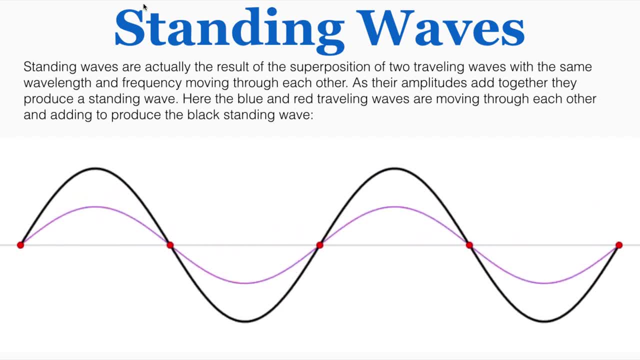 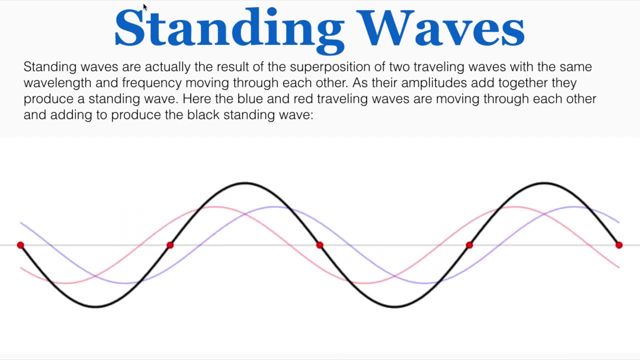 to understanding everything else that happens in this series on standing waves. You have to understand that a standing wave is really just the superposition of two traveling waves moving through each other like this, So I would honestly take just another second to observe the pattern that you're seeing here and 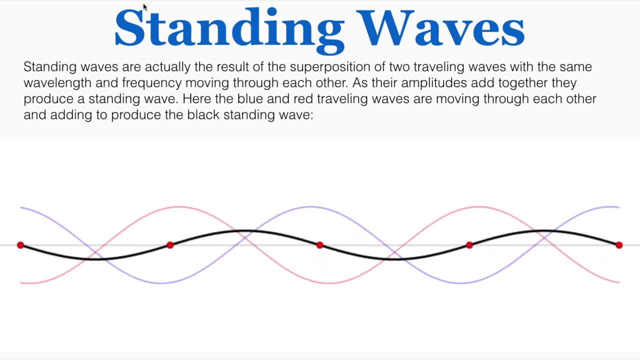 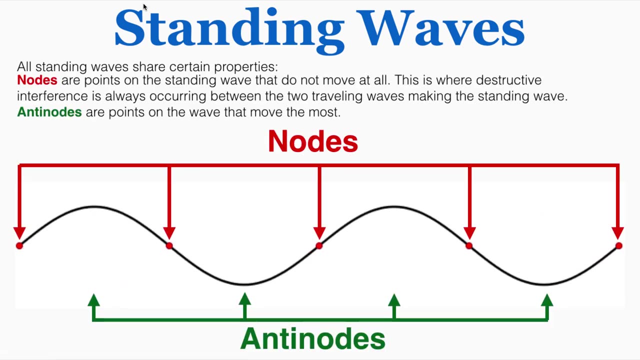 make sure you understand how that standing wave is forming. It's just the sum of the amplitudes of the two waves moving through each other. following the rules of superposition, All standing waves share certain properties. Nodes are point on the standing wave that. 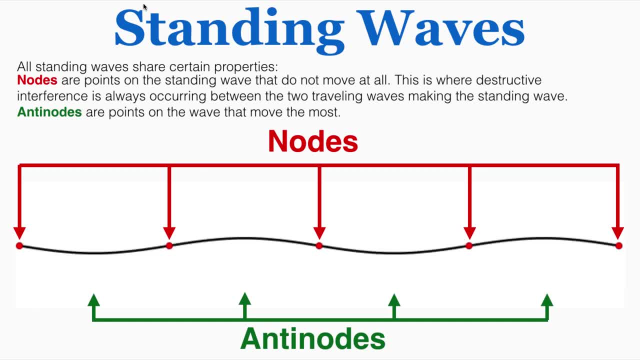 do not move at all. This is where destructive interference is always occurring between the two traveling waves, making the standing wave So at every node, that's the exact point where the two waves are canceling each other out to produce a total amplitude of zero. So those 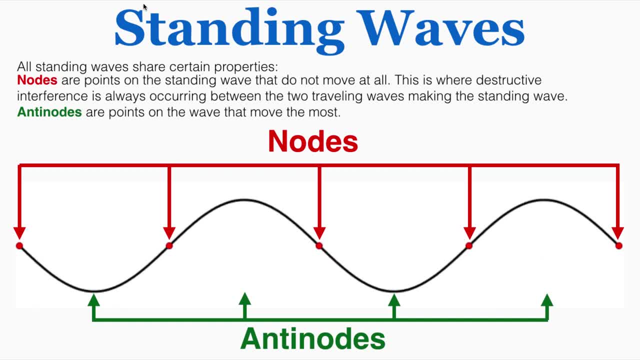 nodes do not oscillate at all. The material in the nodes of a standing wave does not oscillate up or down at all. It just stays in place. Antinodes are the points on the wave that move the most, So the places where it reaches its maximum and minimum displacement are the 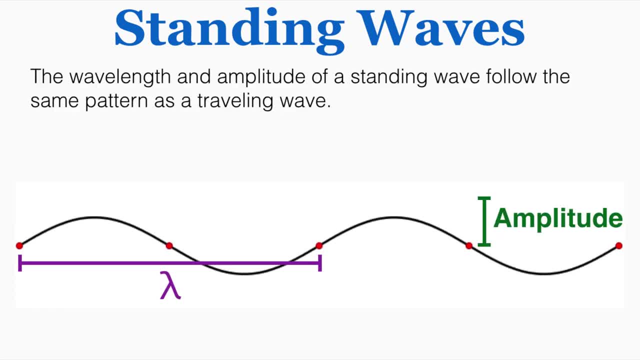 antinodes of the wave. The wavelength and amplitude of a standing wave followed the same pattern as a traveling wave. Sometimes students can get a little confused by the wavelength and assume that the length is just the distance between two nodes, But it's still the length of one complete wave. 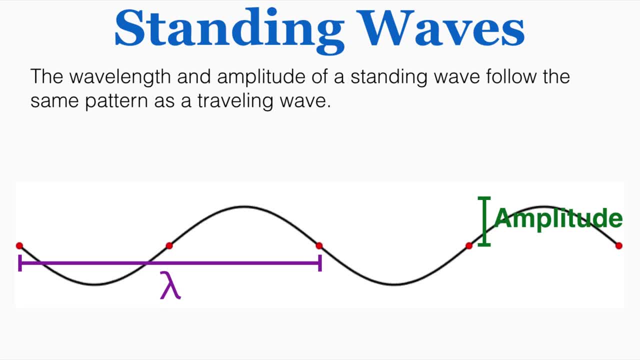 pattern, going all the way up and then all the way down and then back to where it started. So that purple line shows the full wavelength of this standing wave And the amplitude is just from the center point to the maximum point, not from one extreme to the other extreme. 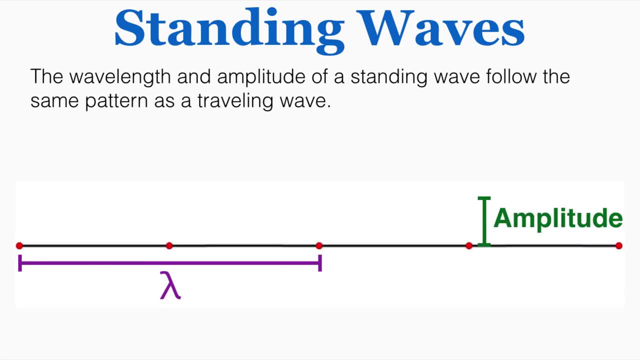 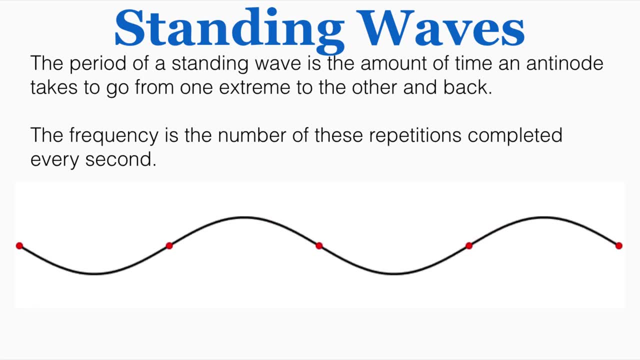 So not from the very minimum bottom of the wave to the very top of the wave. The period of a standing wave is the amount of time an antinode takes to go from one extreme to the other and back. The frequency is the number of these repetitions completed every second. 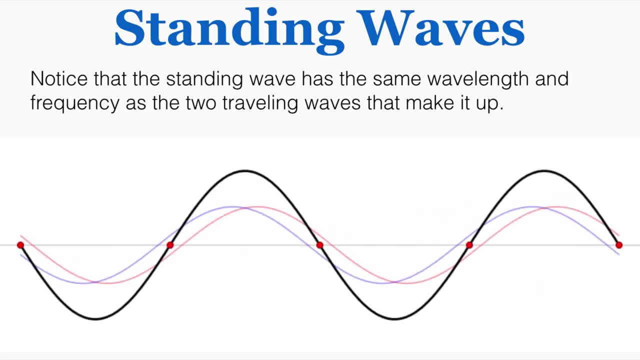 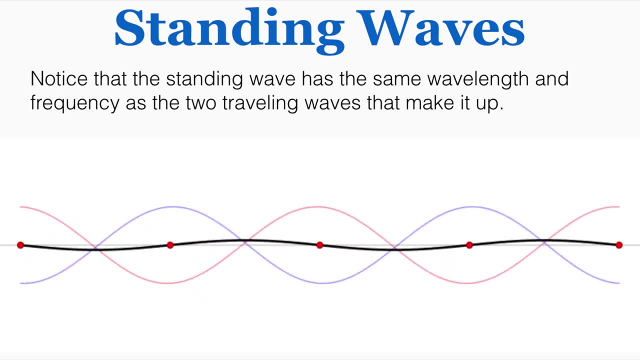 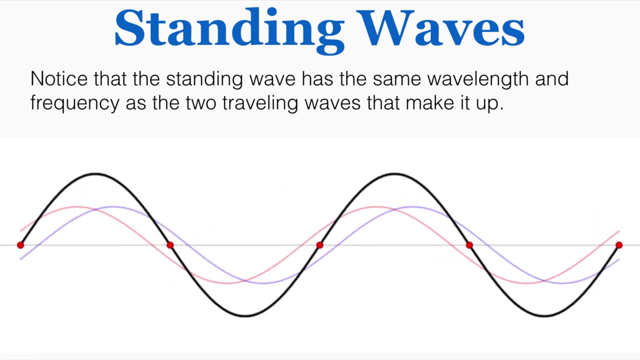 This is another really central fact about a standing wave: It has the same wavelength and frequency as the two traveling waves that make it up. So if you observe how many complete traveling waves pass by a certain point in one second, that's exactly equal to how many oscillations the standing wave makes in one second. 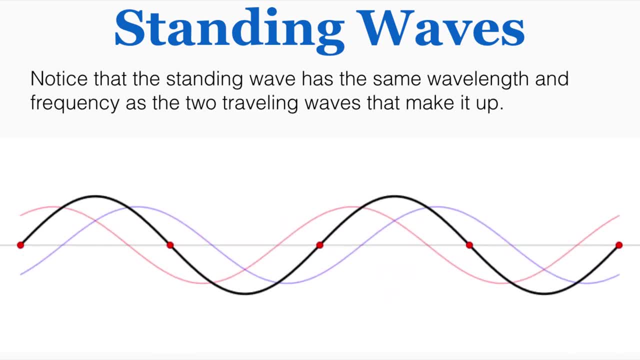 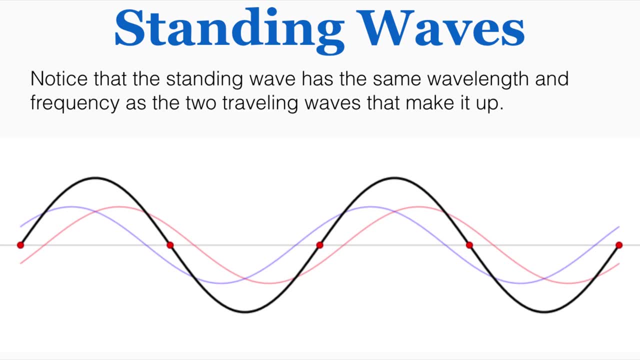 So the period and frequency of the two traveling waves are equal to the period and frequency of the standing wave. If I count the total period for the standing wave, the time it takes to oscillate from the top to the bottom and back, I can count one, two, three, four. 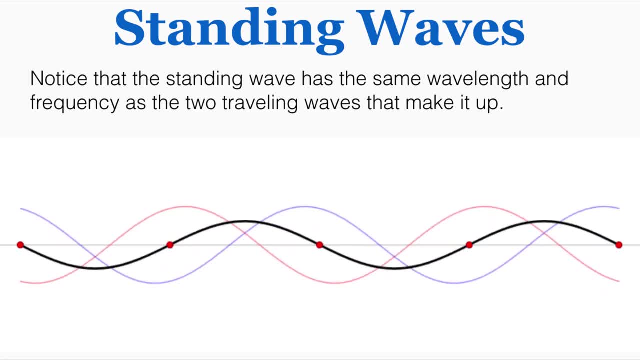 So this seems to have a period of about four seconds, And if I watch at any one point that the traveling wave is moving through and count one, two, three, four, that's the time the traveling wave takes to complete one full motion. 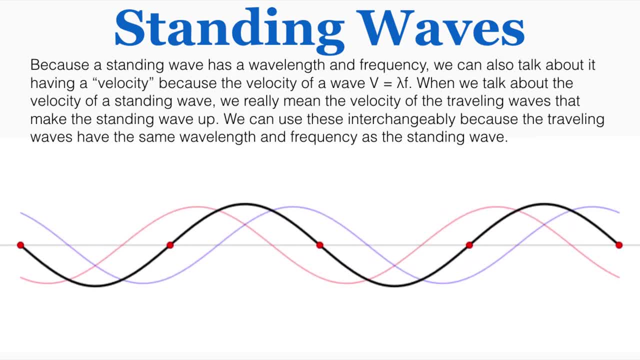 Because a standing wave has both a wavelength and frequency. we can also talk about it having a velocity in quotes, because the velocity of a wave is equal to wavelength times frequency. And when we talk about the velocity of a standing wave, we really mean the velocity of the traveling. 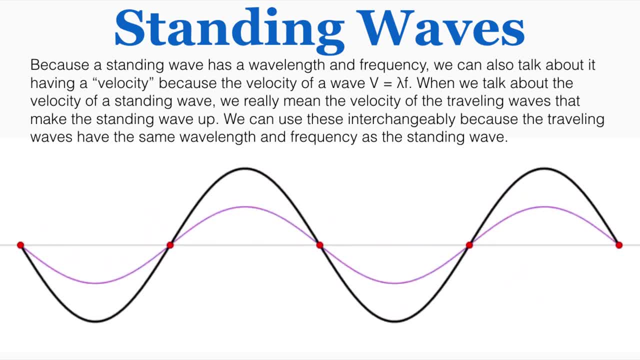 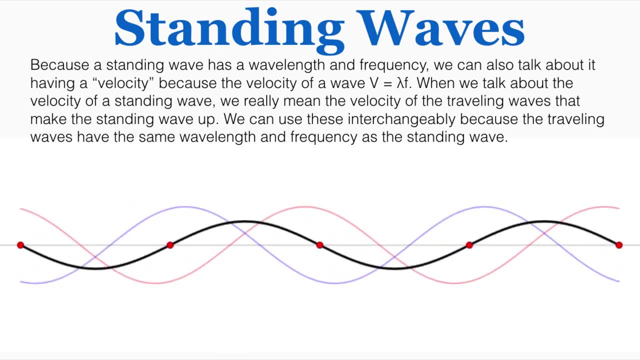 waves that make the standing wave up. We can use these interchangeably because the traveling waves have the same wavelength and frequency as the standing wave. So because the standing wave is standing, obviously it's not standing, It's not actually moving at, say, three meters per second. 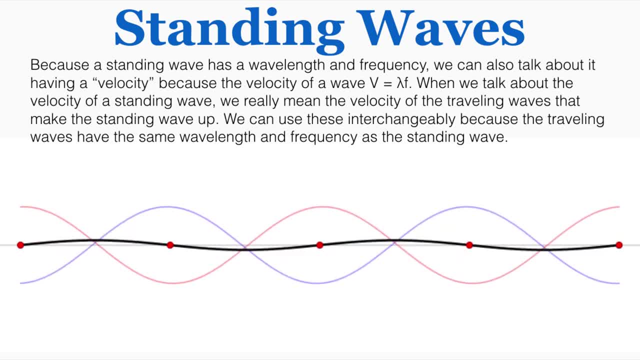 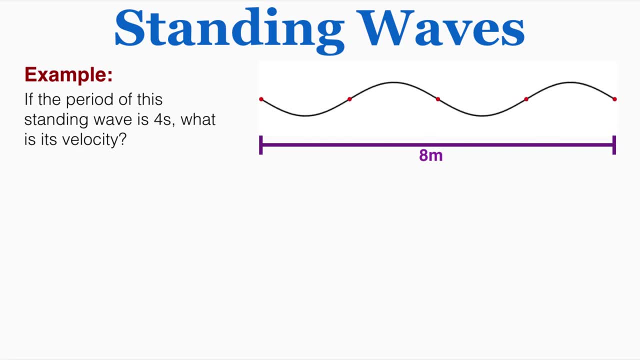 But it can still have a velocity, because when we talk about velocity we can really be referring to the traveling waves that make it up. So, as an example problem, we can ask: if the period of the standing wave is four seconds, what is its velocity? 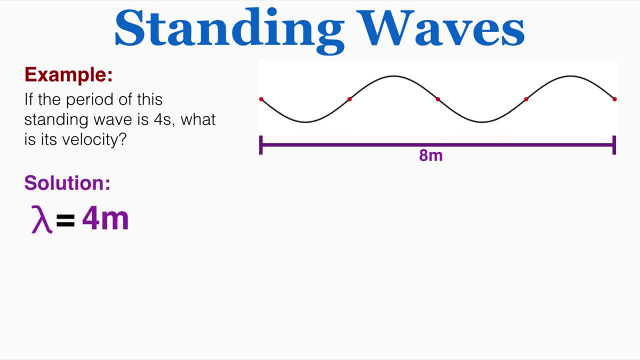 I can see that, because this total length is eight meters, the wavelength is going to be four meters. because that total length is two complete wavelengths. The period is four seconds, Which means that the four seconds is the total length of the standing wave. The frequency, which is always one over period, is equal to 0.25 hertz.